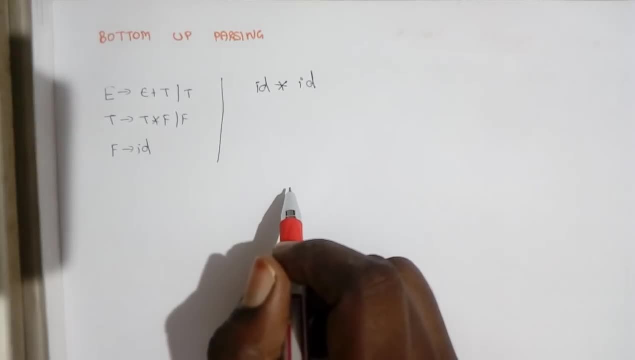 Hello everyone. in this video we will see what a bottom up passing is. A bottom up passing is the reverse of top down passing. We start with the input symbol and we keep on reducing it with its corresponding prediction, and finally it will lead to a starting symbol. 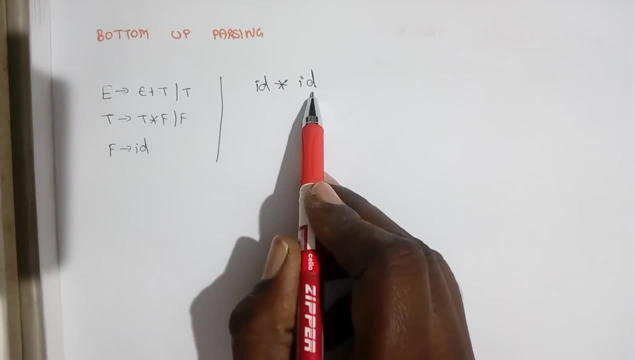 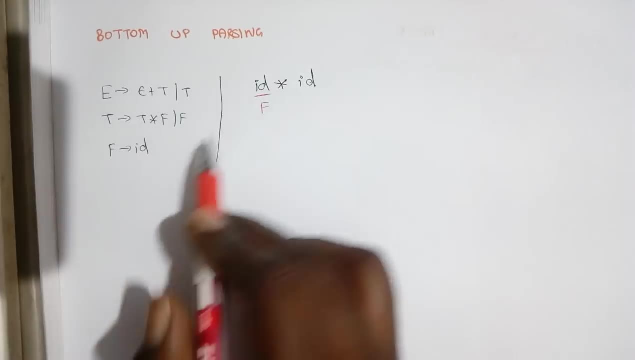 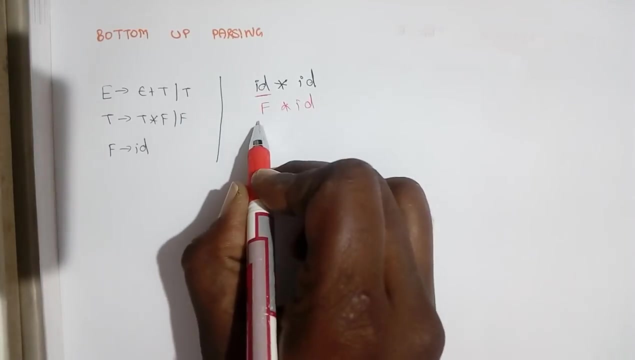 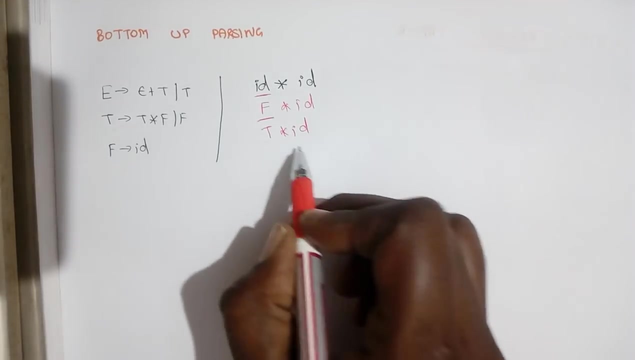 For example, when you consider an input like id, star id, this input belongs to this grammar. So first this id can be replaced with f. Since we have a prediction: f tends to id, we can replace this id to f, and then f can be replaced with t tends to f. We can have t star id, and again this id can be replaced with f. 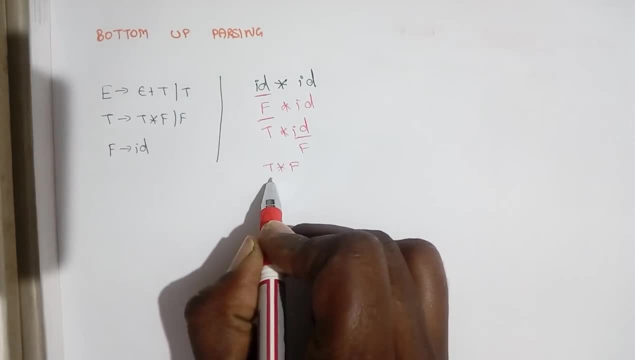 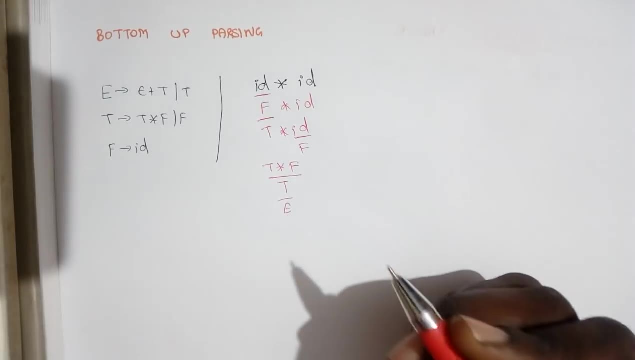 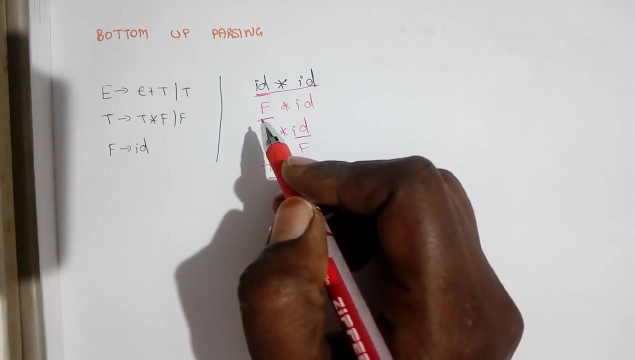 So it will be t star f. And finally, for t star f, it tends to t and we have e tends to t. So we start with this input symbol. We apply one prediction at a time, Like we reduce it. This process is not a derivation, It is opposite to derivation. 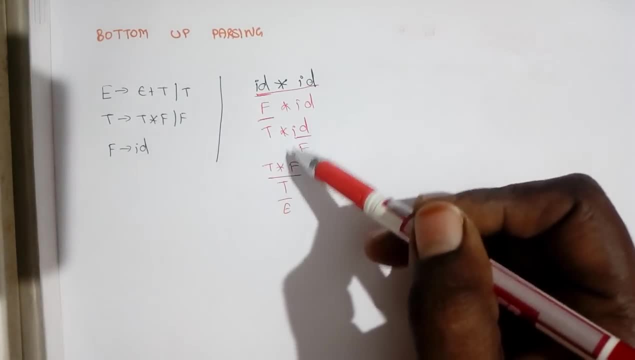 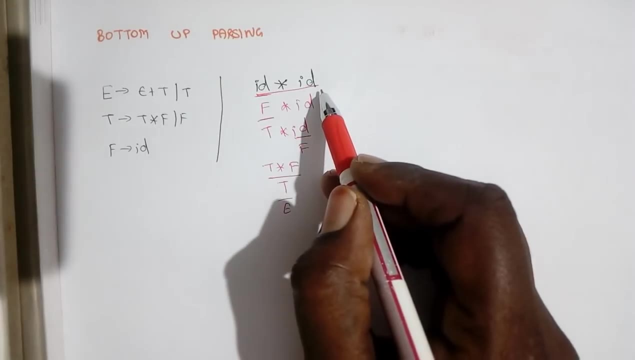 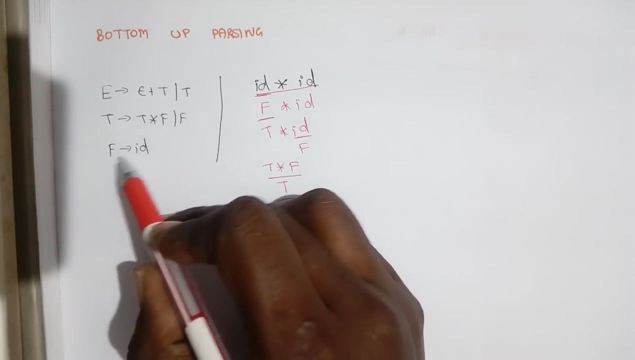 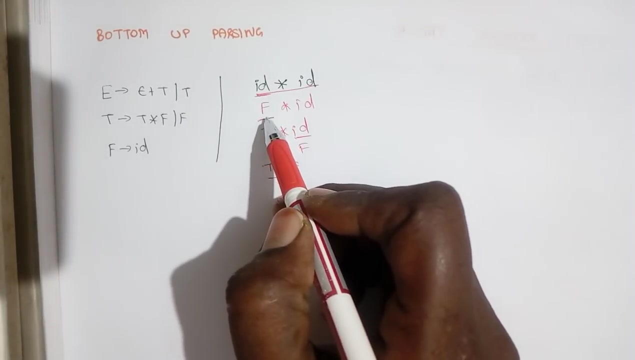 In derivation we start with the starting symbol, We keep on applying some prediction and we derive to input, and this process we call it as reduction. We start with the input symbol. Each step we check the body of the prediction and whichever variable corresponds to that, like it equals to that, we are going to replace that with this variable. So id to t- sorry f- f to t and this id to f, t star f is reduced to t. 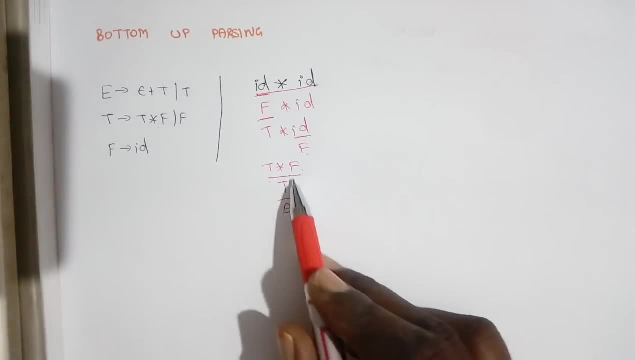 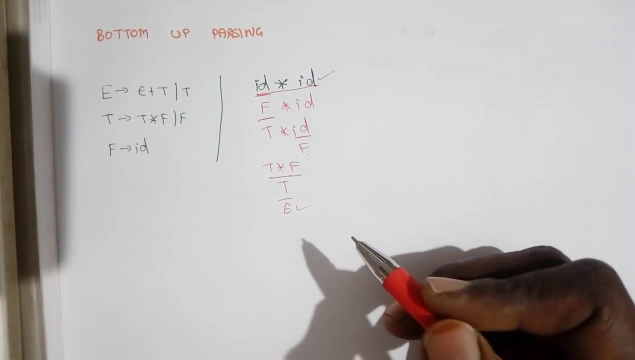 We have a prediction: t tends to t star f, So that is reduced to t. and finally, we got the starting symbol. So we start with the input symbol and when you derive it, derive the starting symbol. We call this type of parser as a bottom up parser. 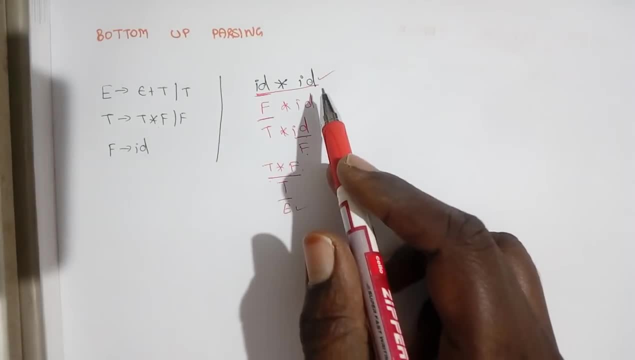 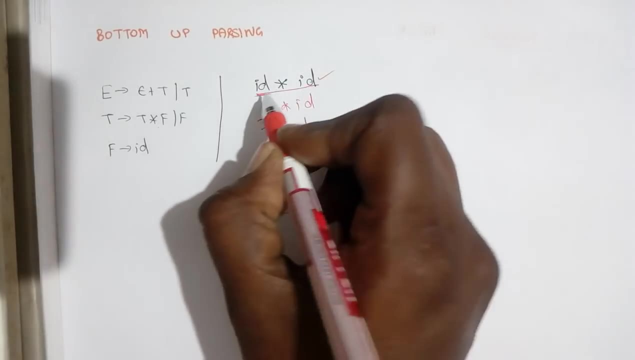 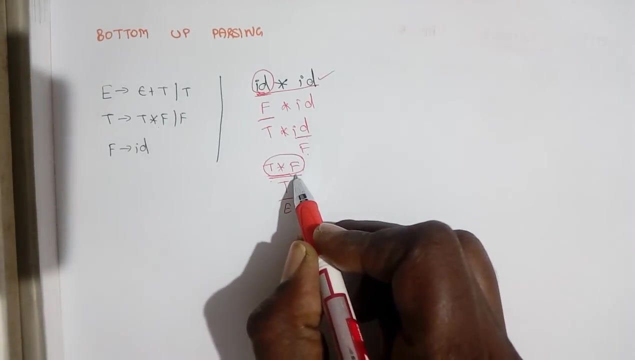 And here we have used reduction process. This process is called reduction In the process of reduction. each time we take a single element or some set of element and we apply this prediction over here, We reduce this to a variable. So this is called handle.